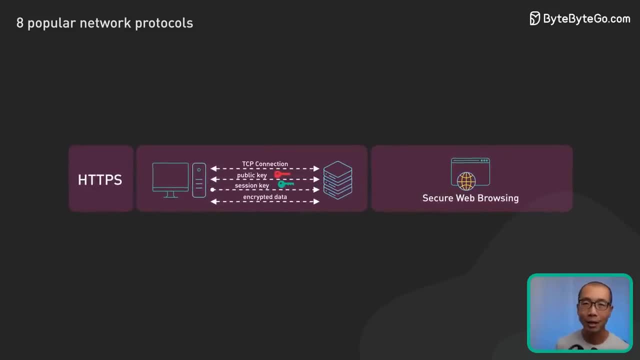 encryption through Transport Layer Security, or TLS. TLS allows the browser and server to make an encrypted connection, like two people agreeing on a secret code. This encrypted connection keeps data confidential as it travels over the public Internet. Traffic is scrambled, so it's meaningless to anyone intercepting it. 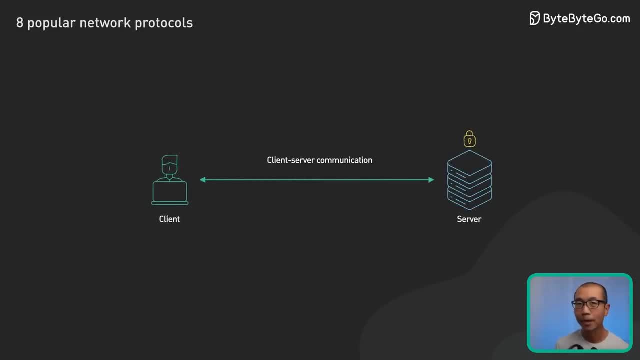 TLS also verifies the server's identity. This prevents crooks from impersonating legitimate sites in what's called a man-in-the-middle attack. So TLS provides the encryption and authentication that powers HTTPS. Copyright-adjusting platforms are verified, and web complaints are clearly false. It's hard to verify that they are fake. OH, it's part of the network's history. This is part of the world's history. 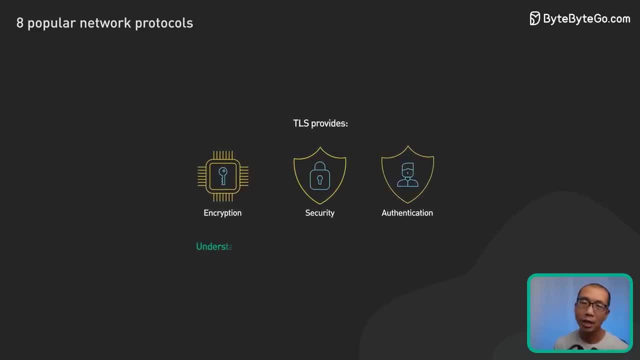 XGTPS and secure websites. Understanding it allows proper XGTPS configuration for safety, which is essential for critical use cases like banking and e-commerce. 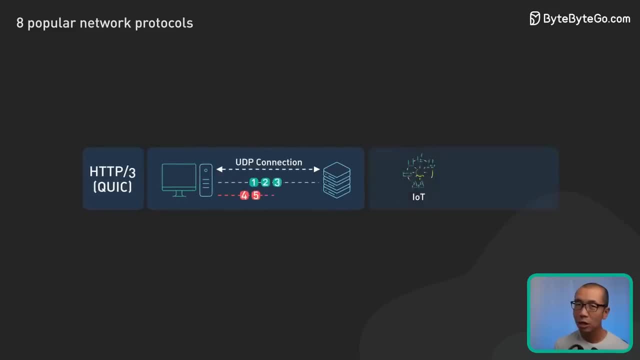 Next up, XGTP3. XGTP3 aims to improve speed and security and fix some nagging performance issues with previous versions. XGTP3 uses QUIC, built on UDP rather than TCP. 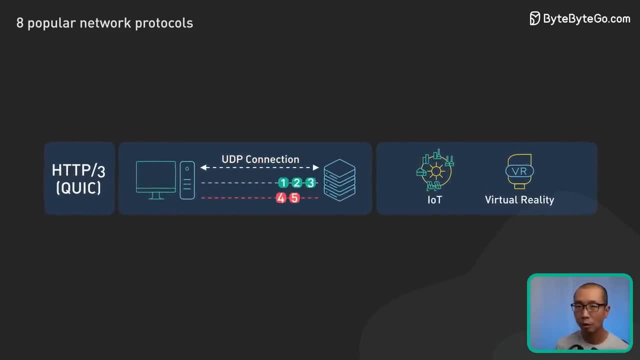 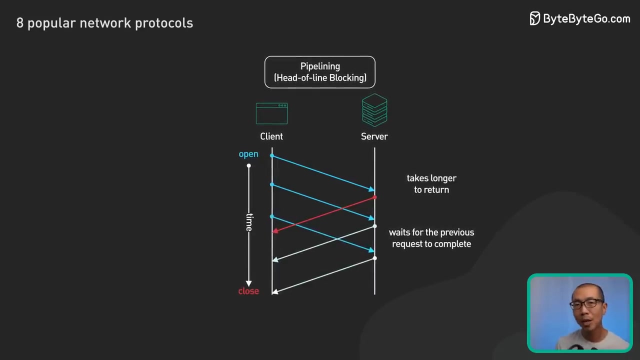 This optimizes performance without TCP overhead. QUIC minimizes lag when switching networks on a smartphone. Leaving the house or office will have less slowdown. QUIC eliminates head-of-line blocking, where one loss packet stores streams behind it. Now other streams don't wait for a store one. QUIC speeds up the initial connection setup. It combines cryptographic and transport handshake into one action. Clients can skip round trips, for servers they've connected to before. This zero-RTT resume is much snappier. 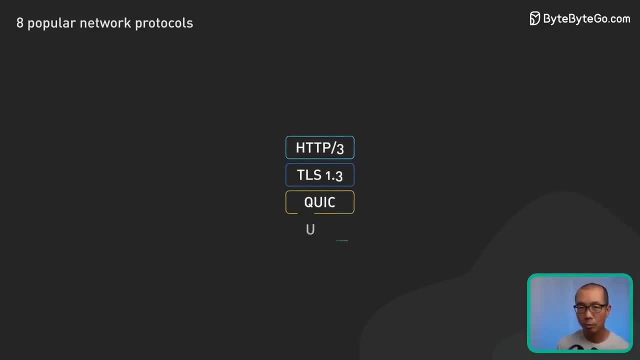 Additionally, QUIC brings encryption by default at the transport layer. All connection data is encrypted, not just the application payload. Even metadata like packet numbers get scrambled. For modern apps, every millisecond counts. 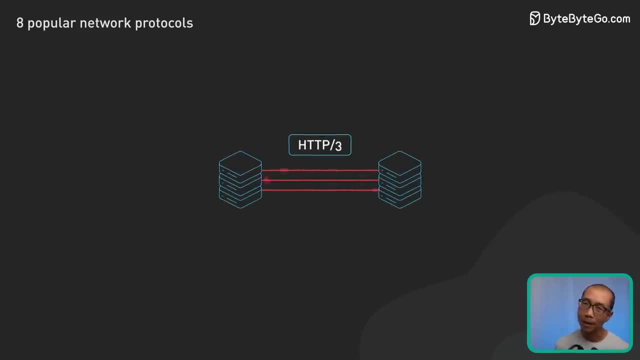 XGTP3 delivers data fast. Shifting to real-time communication, WebSocket is a game-changer. Unlike XGTP, WebSocket provides full duplex bi-directional communication on a single TCP connection. WebSocket enables seamless real-time collaboration and live data streams. The initial WebSocket handshake reuses the existing TCP connection. Then messages can flow freely in both directions with minimal framing. WebSocket supports sending small messages with very low overhead. Ideal for chat, gaming, or real-time updates. Encryption via TLS is supported for security. 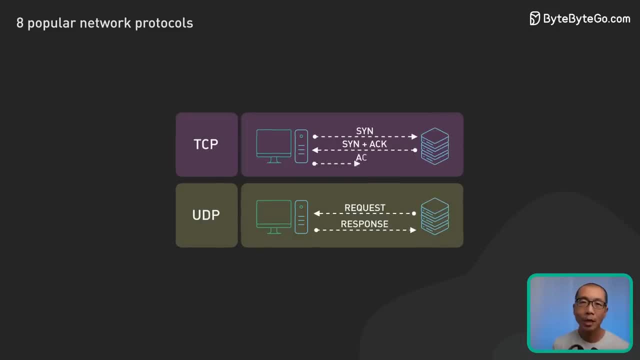 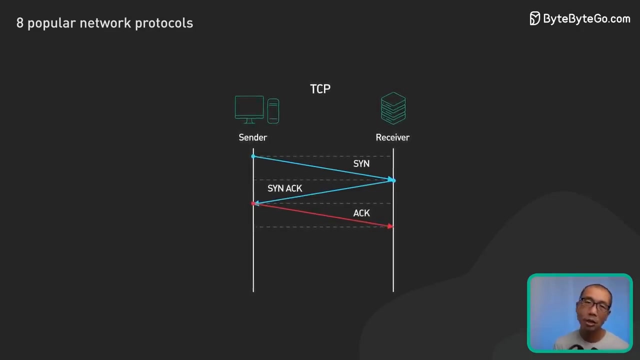 TCP and UDP provide the essential transport layer foundation for many of the application protocols we've covered. XGTP and WebSocket are built on top of TCP. They rely on TCP's reliable transmission, order data delivery, and congestion control to smoothly exchange messages and keep real-time connections stable. 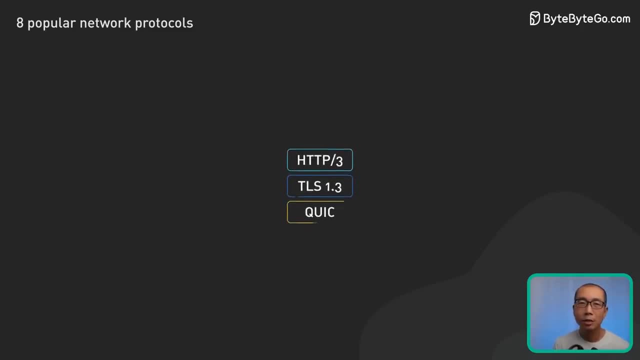 The newer XGTP3 utilizes UDP via the QUIC protocol. This allows optimized performance by reducing overhead compared to TCP. However, UDP lacks reliability, so XGTP3 adds checks to prevent corruption. Now diving deeper, TCP prioritizes reliability over raw speed. Features like error checking, transmission control, and order data delivery ensure robust performance. 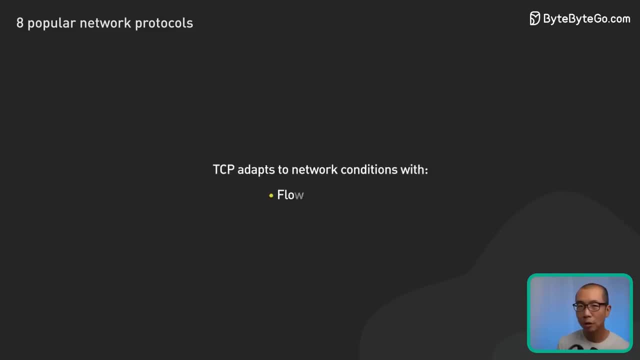 TCP adapts to network conditions with flow control and retransmissions. On the flip side, UDP focuses on speed over reliability. With very lightweight error checking and no handshakes, UDP minimizes overhead for use cases like gaming, voice, Internet of Things, and streaming. 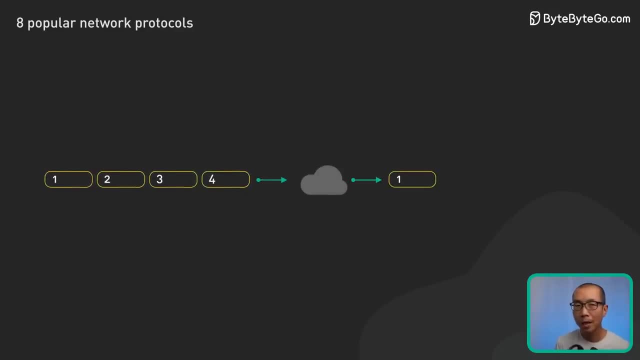 However, UDP data can be corrupted by dropped packets. Combining UDP with application layer integrity checks, balances support, and speed can be a great way to reduce the risk of error. We hope that this video has been helpful. Please like, share, and subscribe! 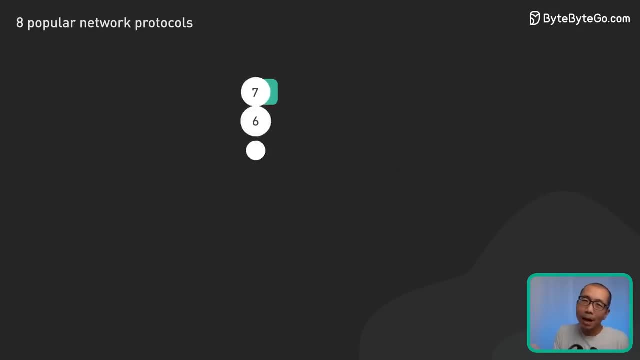 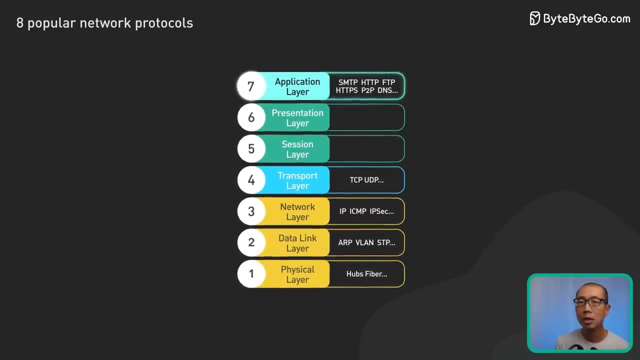 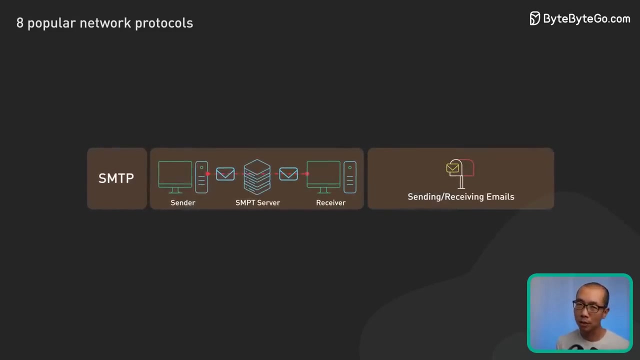 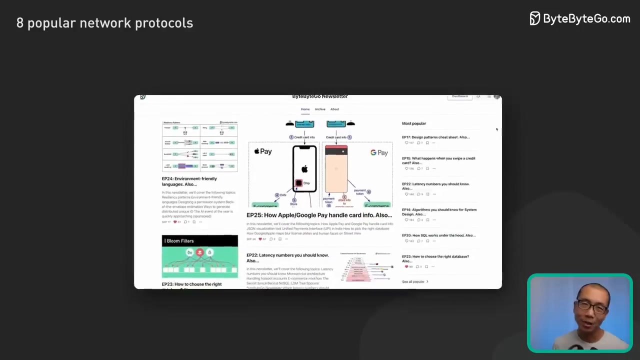 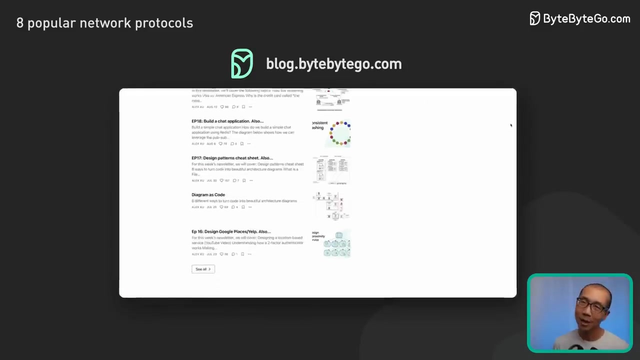 speed and reliability. Now moving back up the protocol stack, SMTP and FTP provide application layer standards for email and file transfer respectively. SMTP is the standard for transferring email messages between email servers. Understanding SMTP helps properly configure mail services and avoid issues like denied listing. FTP allows efficient uploading and downloading of files between hosts. It remains ubiquitous for file-based workflows, especially for financial institutions. Understanding these proper protocols equips us to build fast, secure systems. If you like our videos, you might like our system design newsletter as well. It covers topics and trends in large-scale system design, trusted by 500,000 readers, subscribed at blog.bybygo. com. 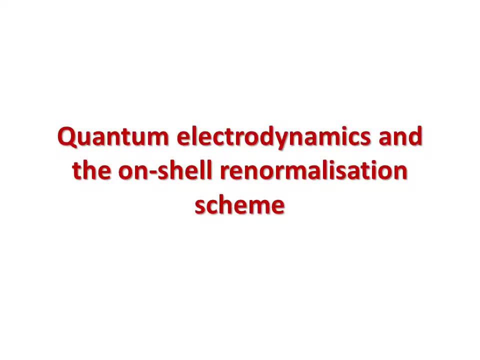 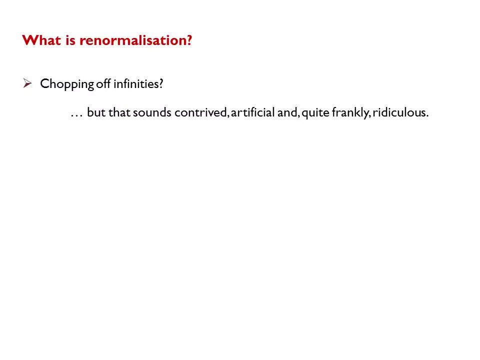 I gave this presentation in Cambridge in January 2013. It was a part of a seminar series for graduate students. The talk is about renormalisation, a concept in quantum field theory that people find disconcerting, and the purpose of the talk is to make it seem reasonable. Let me start by saying what renormalisation is not. It's not a random and artificial attempt at chopping off infinities. A serious physical theory doesn't need that. Some people associate renormalisation with the idea of quantities flowing with an energy scale. It may be helpful to think in this way, but this idea of flow is just an artefact of a particular accounting procedure and it doesn't really get us to the bottom of the issue that bothers us, which is the issue about the infinities in quantum field theory. 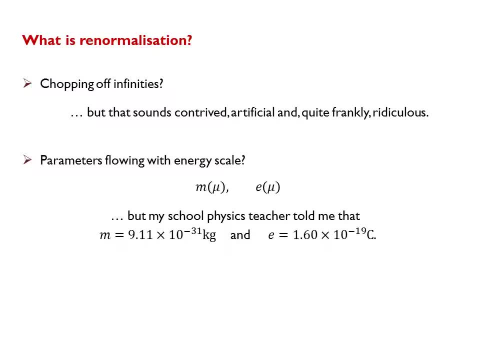 In fact at school, we were taught that parameters like the mass of the electron or the electromagnetic gauge 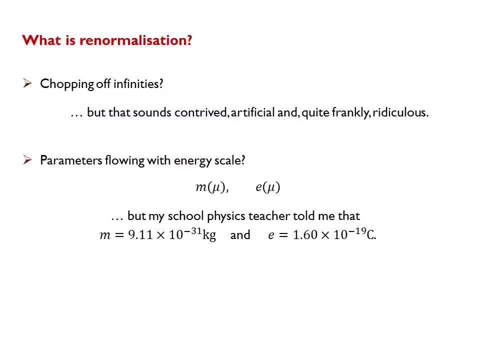 coupling take fixed values, and it's hardly unreasonable to want to present quantum electrodynamics observables in terms of those fixed parameters that we are so well acquainted with. 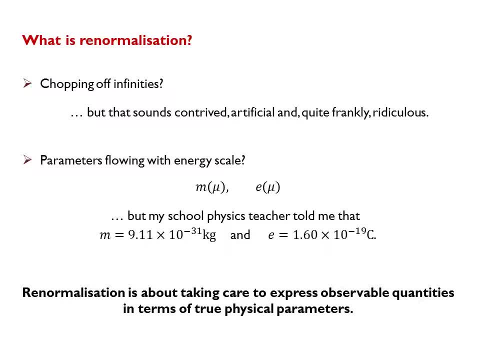 I am going to put forward the view that renormalisation is a natural and inevitable part of doing a field theory calculation. Renormalisation is about taking the care to express observable